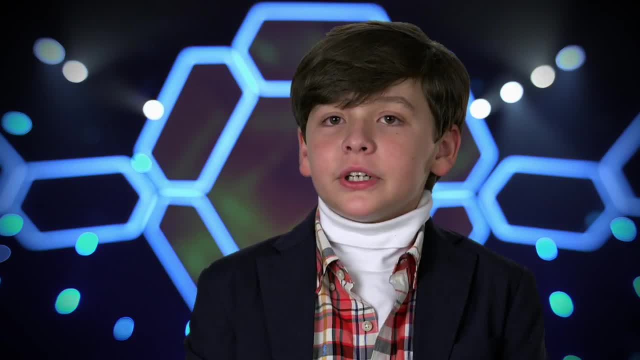 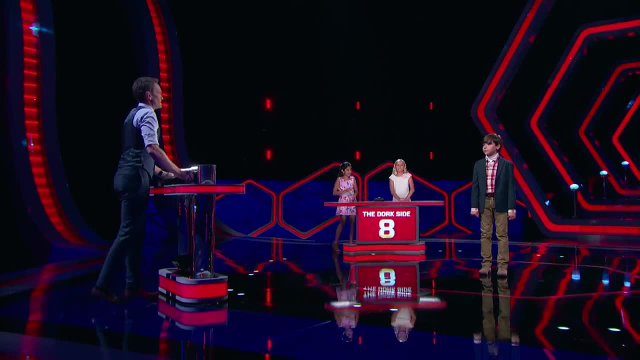 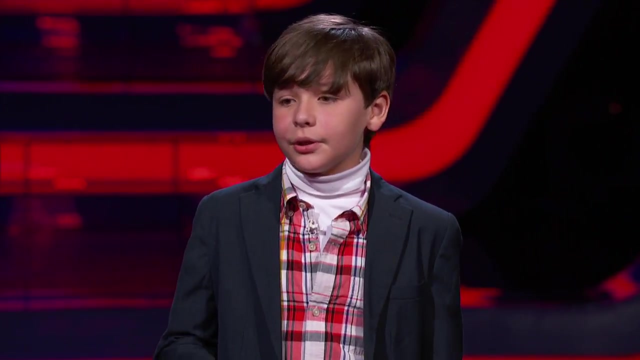 for a normal person there would be a brain crushing amount of pressure. Ah, see what I did there, Rodrigo. why did you choose the super brain? Math is easier for me than everything else, so I'll just do it quicker, Nice. 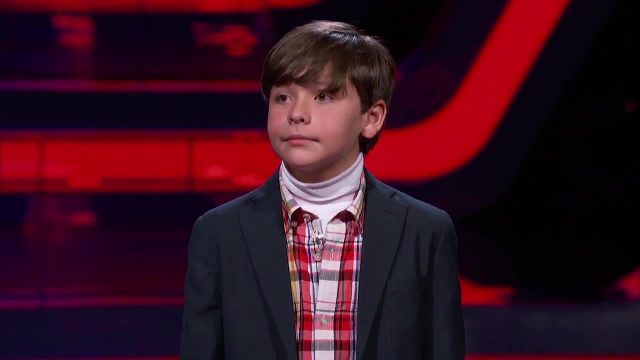 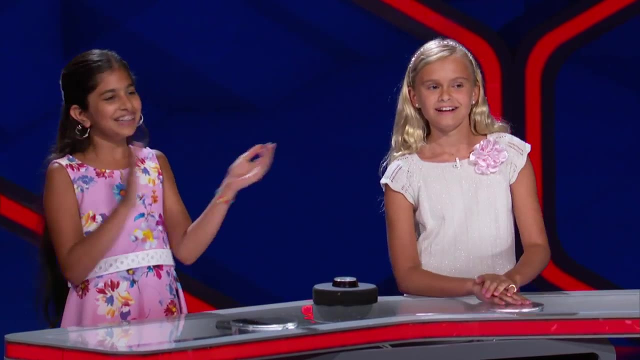 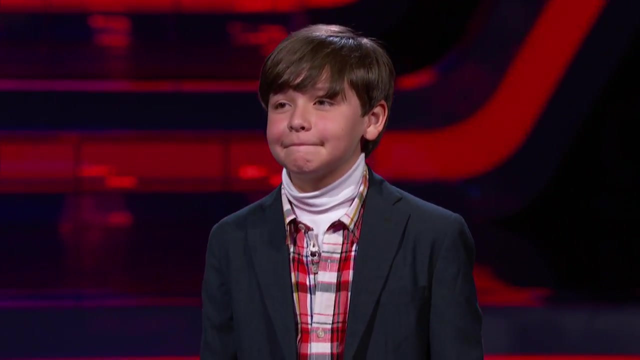 Fingers crossed, Fingers crossed, Fingers crossed- All right, The only thing that's riding on this are your two teammates who are staring daggers at your back. Yeah, but they always do that. Oh My feeling. All right, Let's play number cruncher. 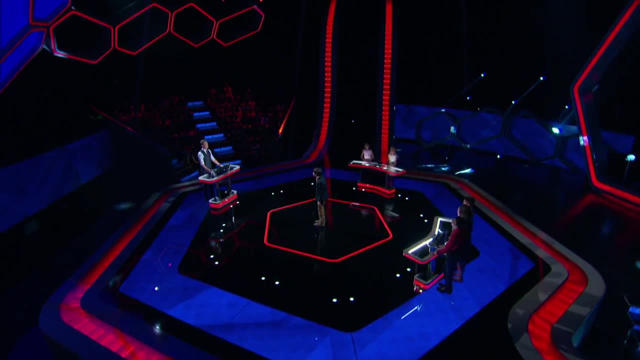 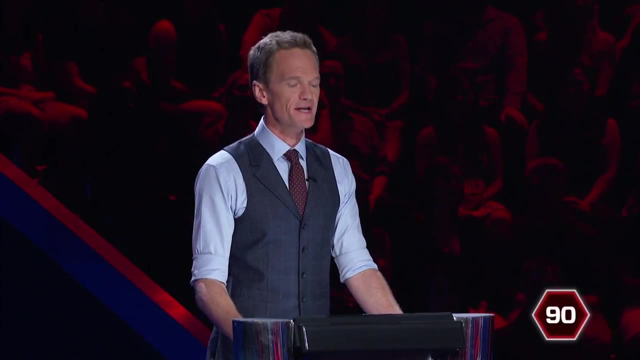 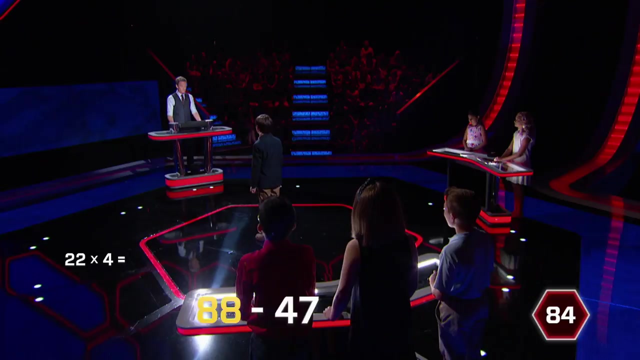 Yay, Remember, you won't be able to see any of the numbers. Rodrigo, you have 90 seconds. Your time starts Now. 22 times 4 equals 88. Correct: 88 minus 47 times 3 equals. 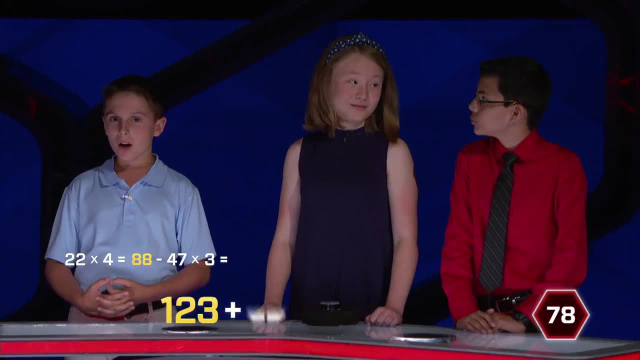 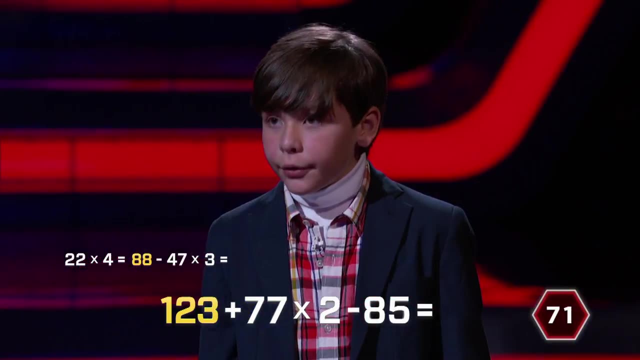 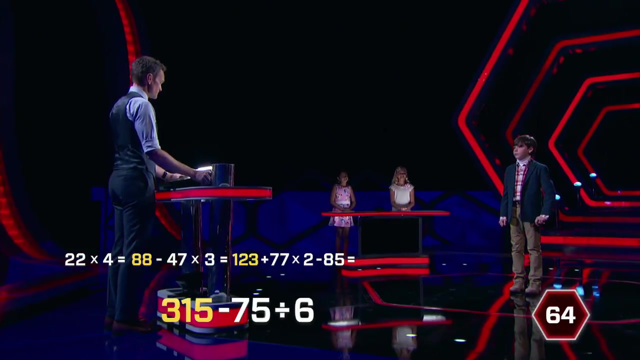 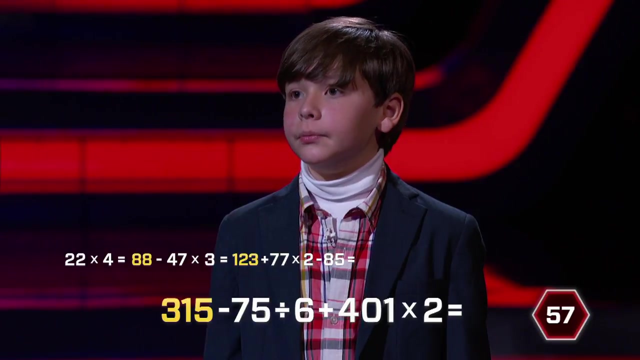 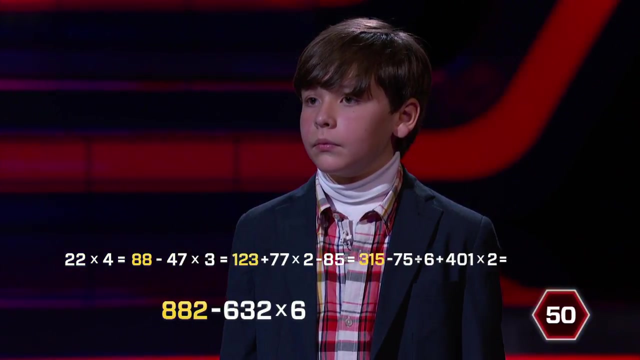 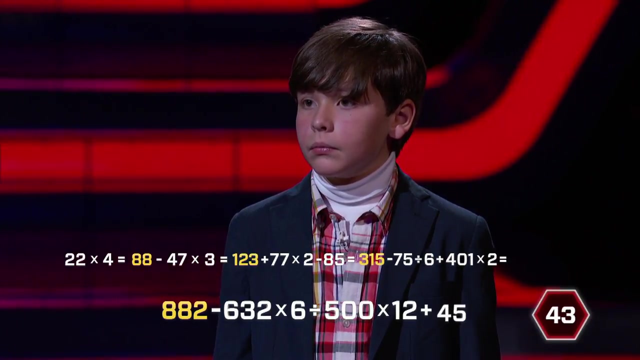 123.. Correct 123 plus 77 times 2 minus 85 equals 315.. Correct 315 minus 75 divided by 6 plus 401.. Times 2 equals 882.. Correct 882 minus 632 times 6, divided by 500 times 12 plus 45, equals. 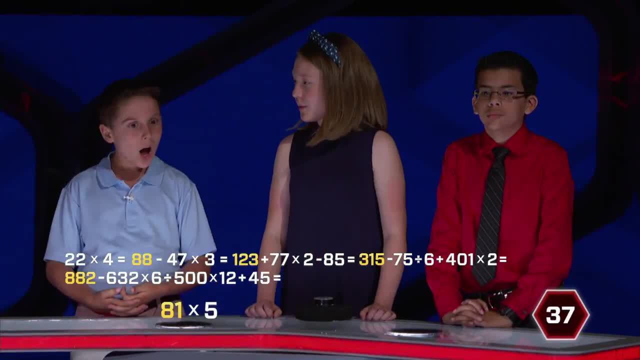 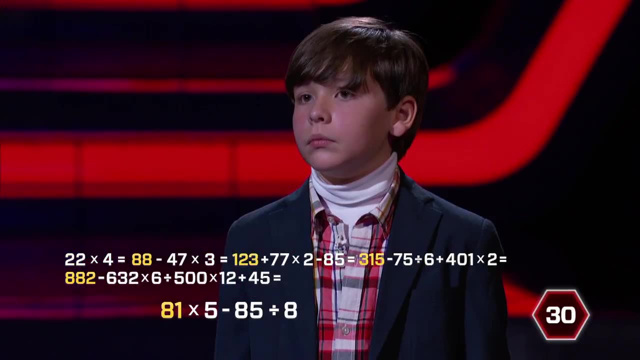 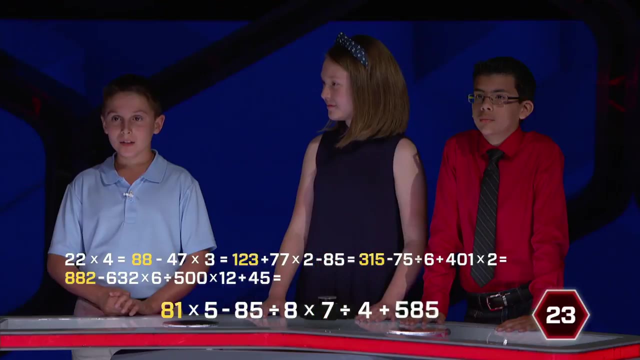 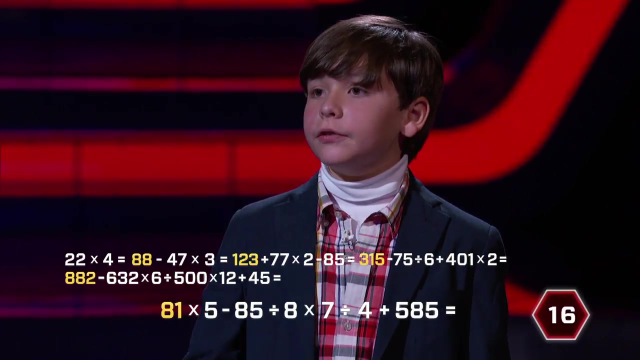 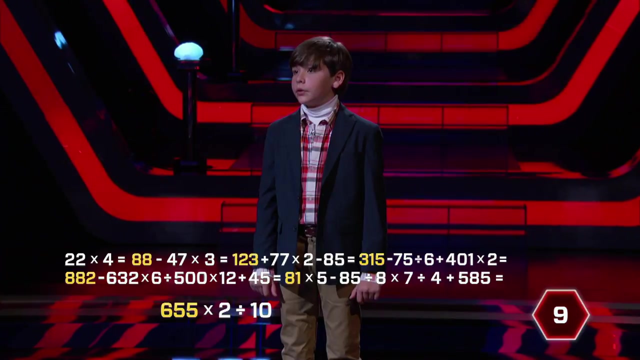 81.. Correct: 81 times 5 minus 85 divided by 8? 8.. Times 7 divided divided by four plus 585 equals 655.. Correct: 655 times 2 divided by 10 minus 50 divided. 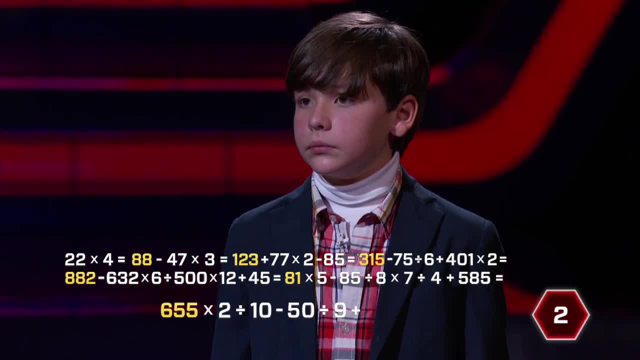 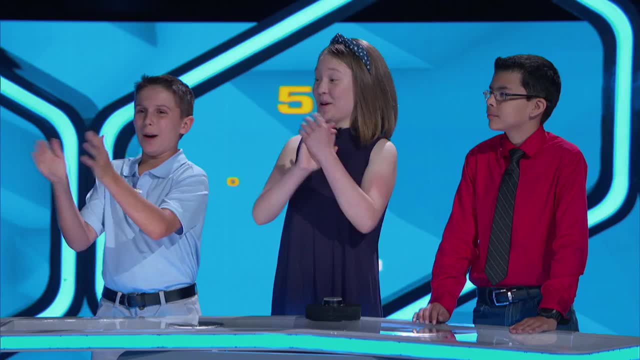 by 9 plus 35.. 655.. 255.. Not an answer. Not an answer. An answer: 650.. 30%, 60%, 37%, 36.. Oh, and time is out Just unbelievable. 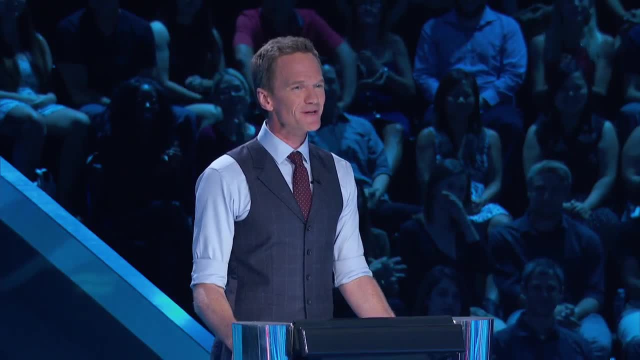 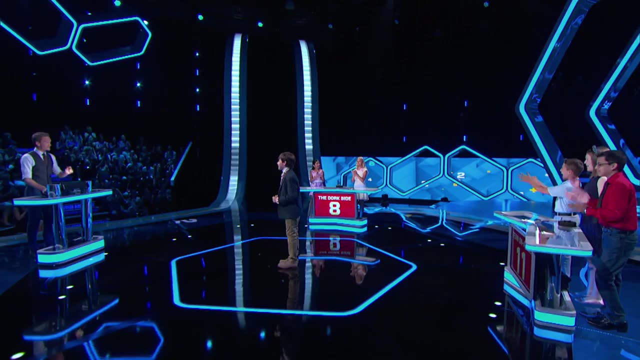 Amazing. I think you guys made a terrific choice in having you be the super brain. You crushed it. You got six answers correct for a total score of 14.. Head on back to your podium. I'm going to crush them this time, though. OK, you are amazing, You are amazing. 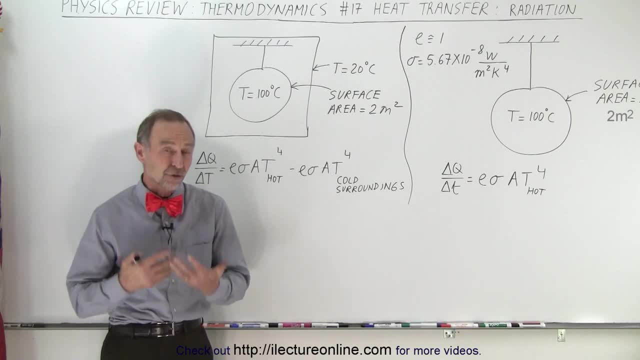 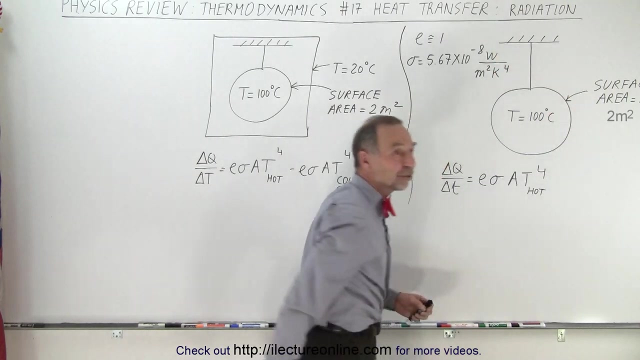 Welcome to iLecture Online. The next type of heat transfer we're going to review is radiation, And that one is typically fairly straightforward, So we're going to take it in two steps. The first step is that we have just an object that's radiating out and we do not care about what's. 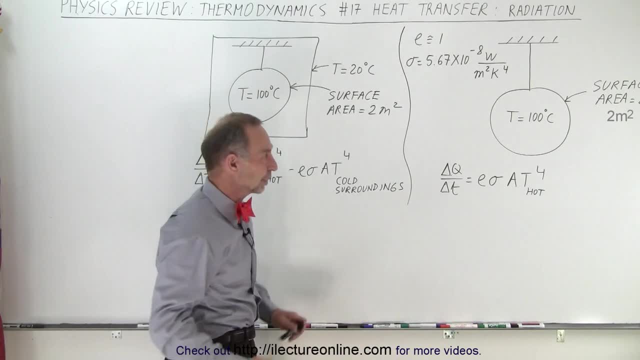 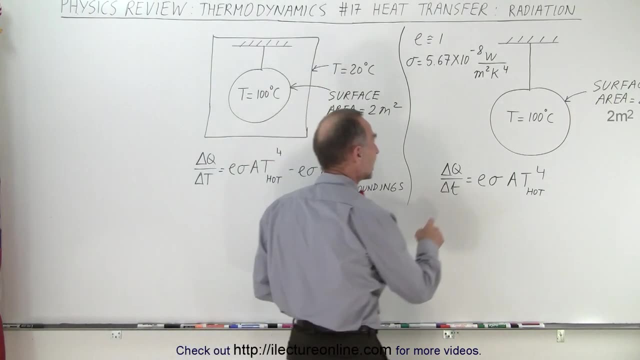 around it, Empty space at zero degrees Kelvin. We don't care. So there's only radiation going out and there's no radiation coming back. And so that way we can say that the amount of radiation that gets radiated, the amount of heat that gets radiated, is equal to the emissivity which we 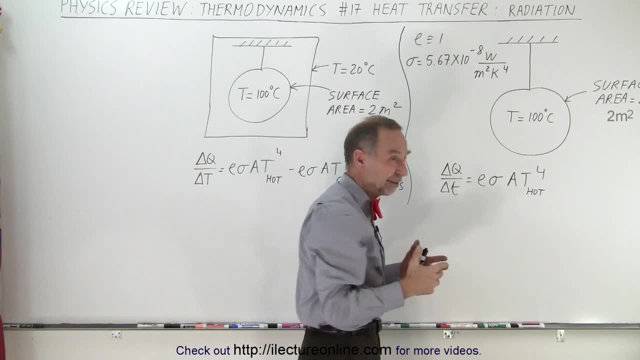 typically say it's about one. There's some exceptions to that, but for most materials it's close to one. This is the conductivity constant. So not conductivity constant, but this is sigma. This is the radiation constant. we need Sigma 5.67 times 10 to the minus 8.. This is the surface. 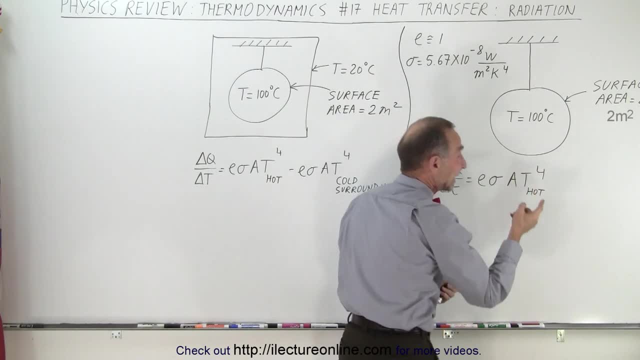 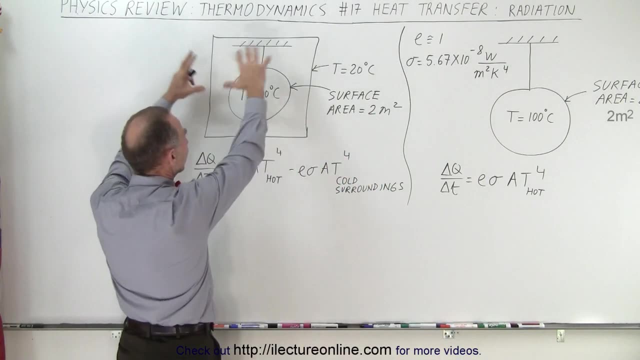 area of the object that's radiating and then the temperature of the object in Kelvin. So we have to convert to Kelvin, to the fourth power, If we have an object that's surrounded by, let's say, a room that has walls, and the walls are at a 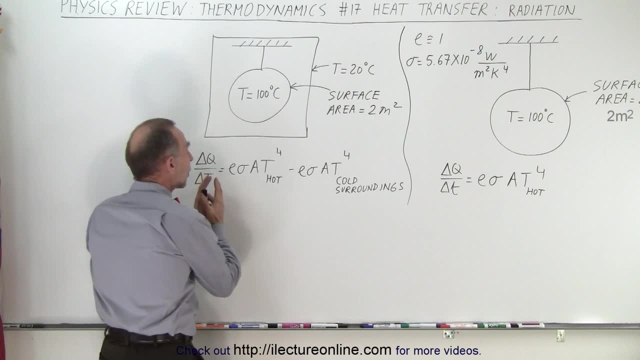 temperature of 20 degrees Celsius, then not only does radiation go out, but it also receives radiation from its surroundings. So the net radiation going out will be what's radiated by the object minus what's coming back from the surroundings. So we'll do it both ways. Now all. 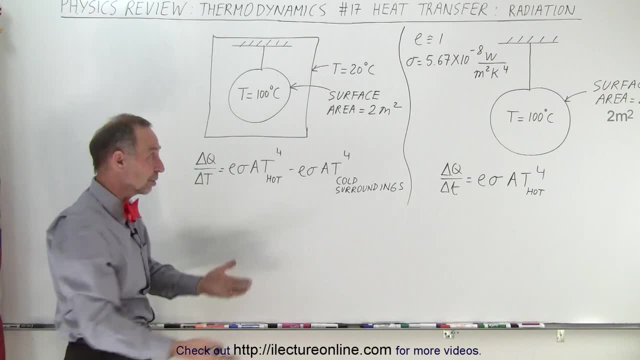 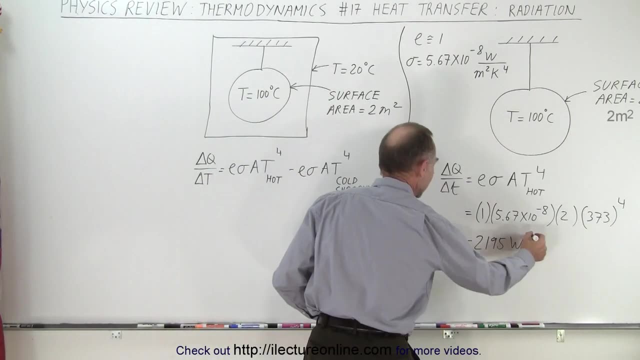 we have to do at this point is essentially: the problem is solved. You have the equation, you plug in the numbers, but that's just the algebra portion. So we'll see what the results will be. The amount of heat radiated per unit time from the hot. 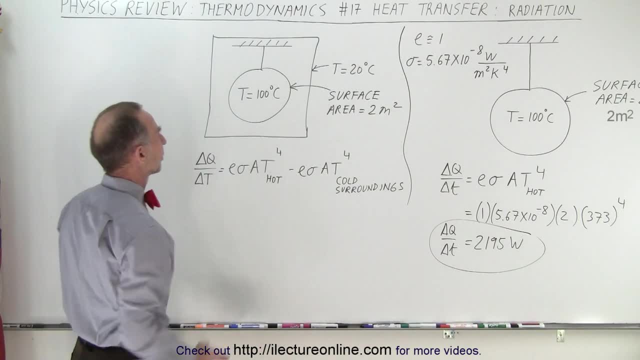 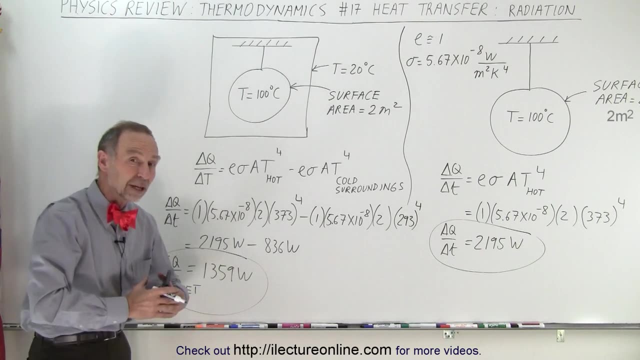 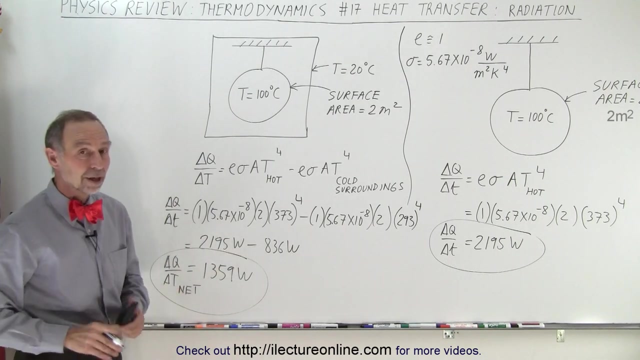 object. So what does it look like when we have the surroundings as well? Radiation, in other words, that is the radiation given off minus the radiation it receives back from the surroundings. So the net loss will be 1359 watts. but if it's somewhere in the middle of nowhere, in the middle of space,